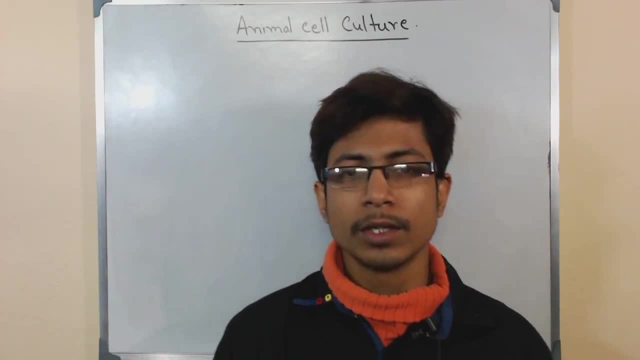 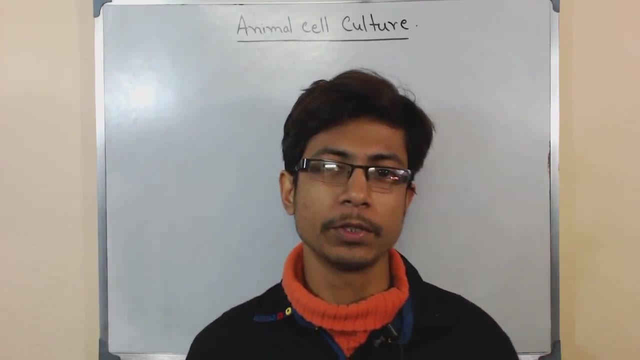 Welcome back guys. Welcome to a new session from Shomus Biology And from now on, in consecutive videos, we'll be talking about animal cell culture, And this is one of the topics that I've been getting more requests from different students. But let's start making videos on. 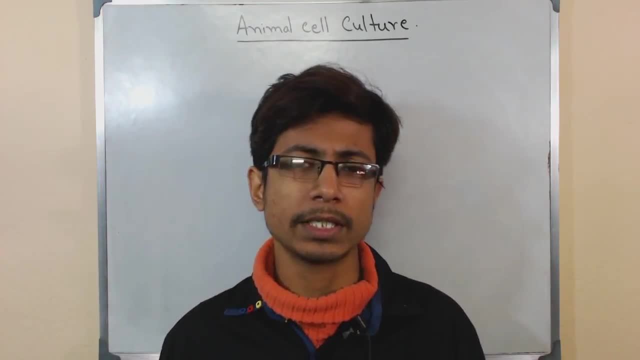 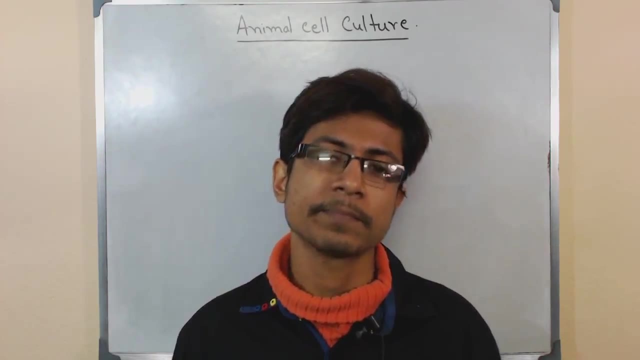 animal cell culture, because this is the part which is not really exploited till now from Shomus Biology and from any other YouTubers or YouTube video providers. So let's begin with animal cell culture. In this whole set of videos, we'll be talking the basics of. 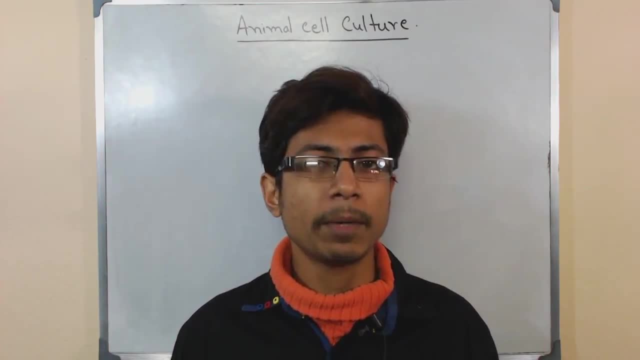 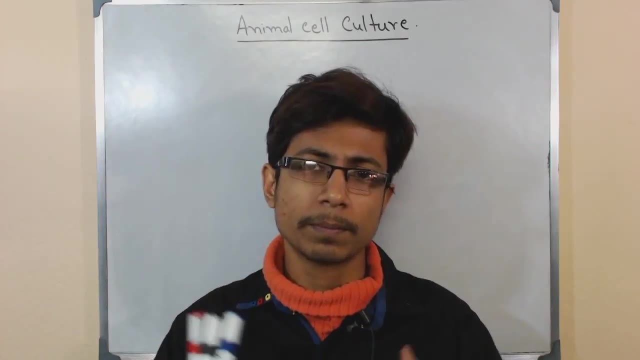 animal cell culture. I am again telling you I'll be talking only about the basics, That means the ABCDs of animal cell culture. I'm not talking about those practical aspects of animal cell culture now. For now on we'll be talking and only understanding the principles. 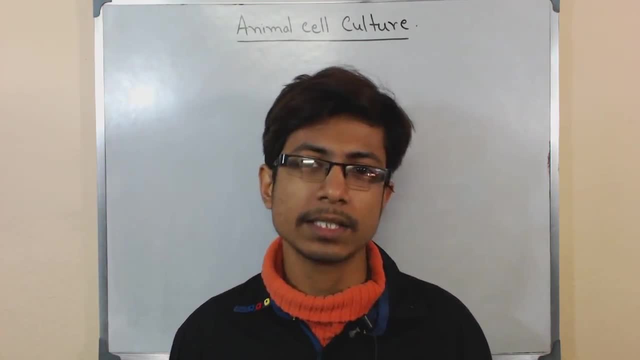 of cell culture, What is going on in inside, Why cell culture is important And what are the different terminologies of cell culture And what are different types of cells. And, more importantly, about certain part of the practical cell culture, that is, a media and their growth and all this part, Okay. 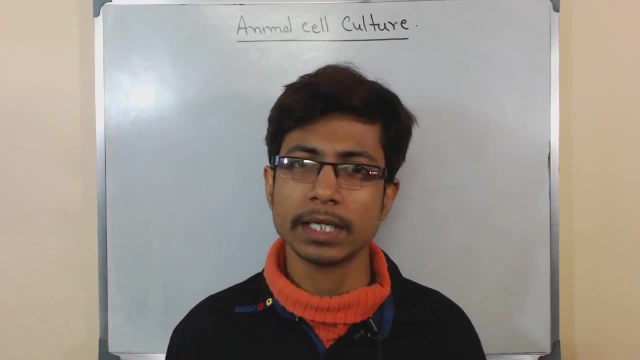 so let's begin with this first video. This is going to be the introductory video about cell culture and cell culture or tissue culture. Whenever we talk about cell or tissue culture, that thing are kind of you know, related They are, they are kind of very same in many. 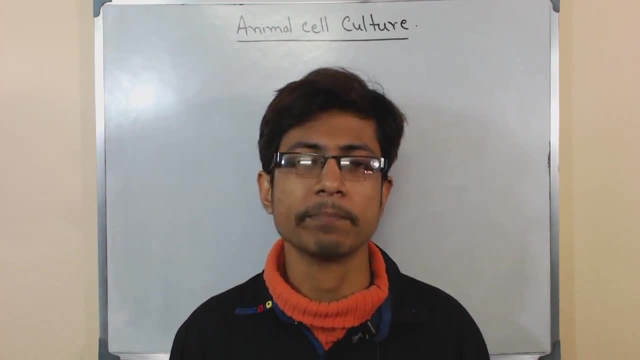 aspects. Actually, there are many important similarities between them. Now, in that case, it can be plant or it can be animal. We have videos on plant tissue culture. You can see all those videos on plant tissue culture in my YouTube channel. You can go there. see a lot of videos. 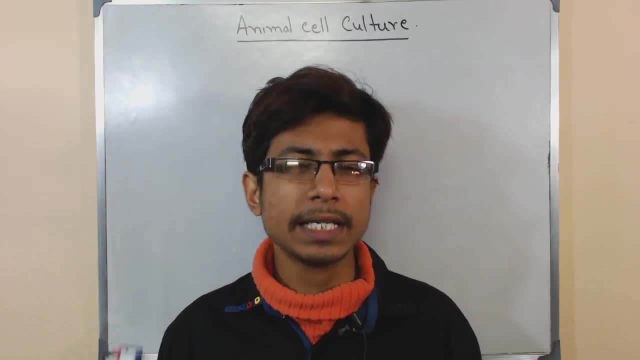 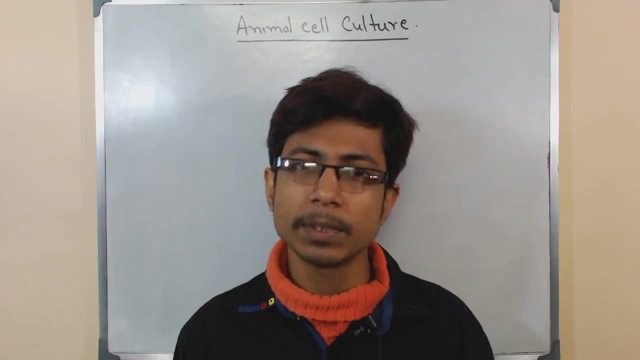 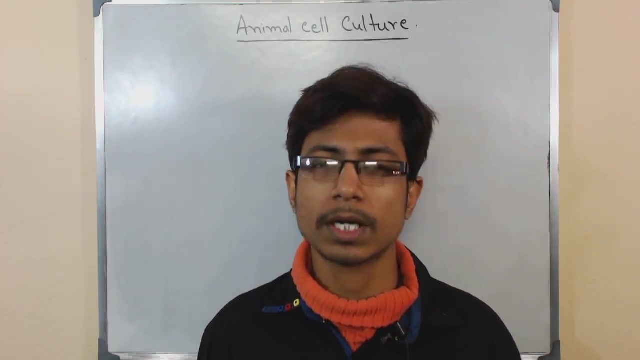 on plant tissue culture are there, but the animal tissue culture is different from plant tissue culture in many ways and you'll be talking about those differences here and also other terminologies. to start with, So far, for the first thing, that the animal culture or animal cell culture that we are going to talk about, animal meals in 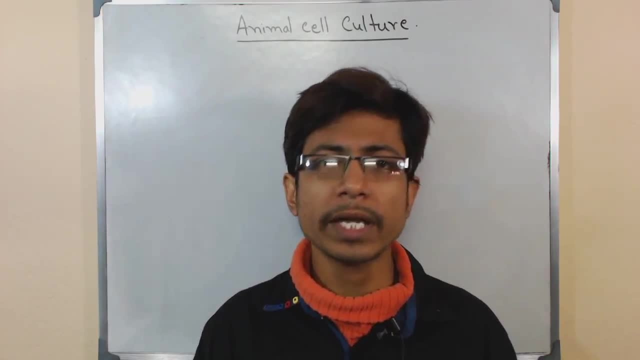 this case we mean eukaryotic animals, because prokaryotic cell culture is easier. it's simply the prokaryotes means morely discovered by bacteria and the bacterial culture. we have already talked before about bacterial culture, how to culture it and all the different aspects of microbiological processes, but in this 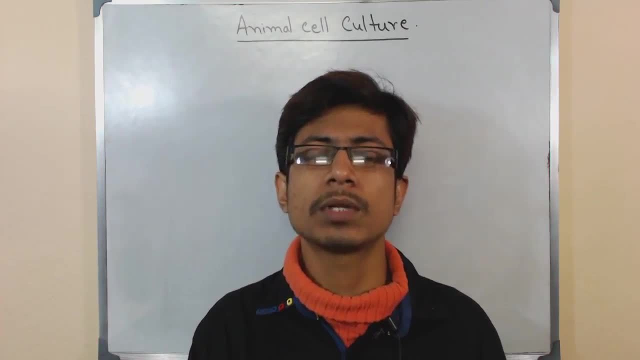 case, animal tissue culture, that is, the eukaryotic animal tissue culture, is far more complicated than the prokaryotic cell culture because, you know, eukaryotic cells have much more complicated cell morphology, they have much more complicated requirements for their growth. so for all these reasons, we need 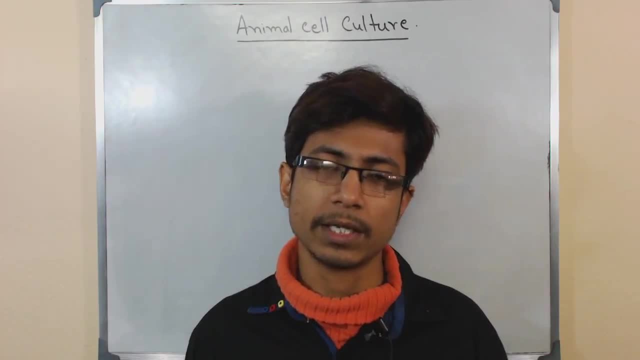 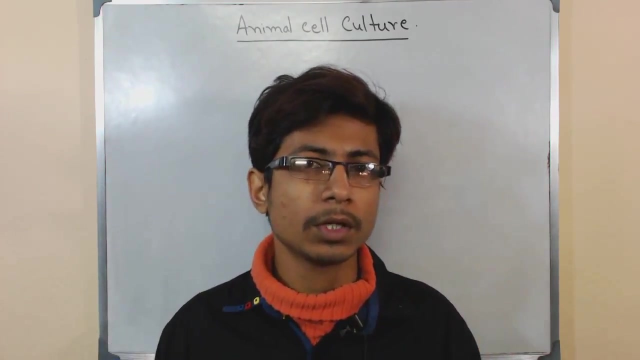 to be very careful to talk about this animal tissue culture, their animal cell culture. it is much more complicated, it is much more vulnerable to contaminations and so that we need to, you know, prepare all these things for beginning. now for the first thing, or first for the beginning. we must know some terminologies about the animal tissue. 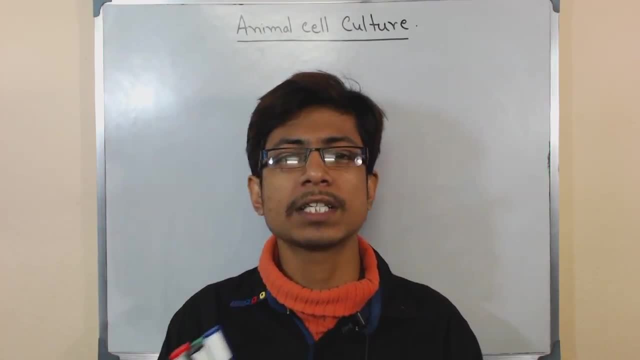 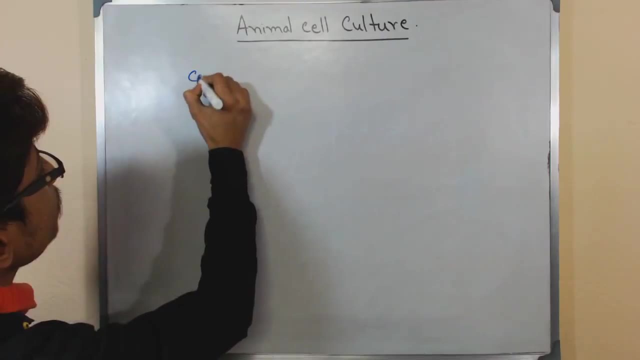 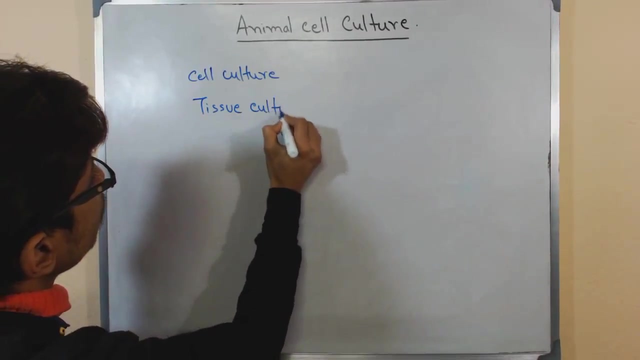 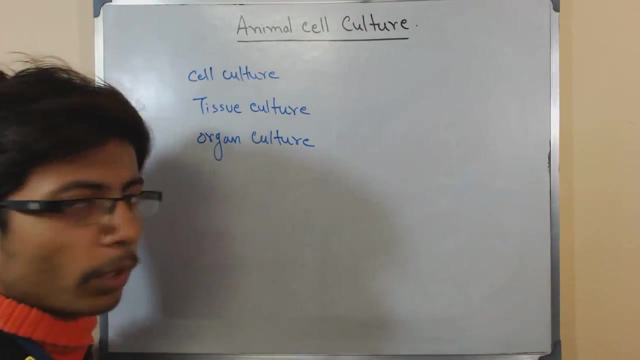 culture and cell culture. that is what is tissue culture, what is cell culture, what is organ culture, because these are the three things that you are going to see coming again and again. so you know, cell culture is there, tissue culture is there and organ culture is also there. you know, the names are kind of very important. 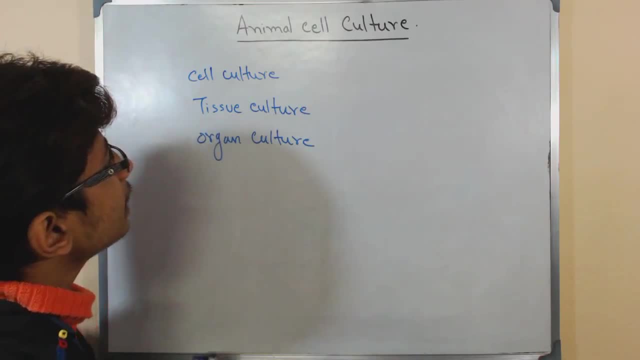 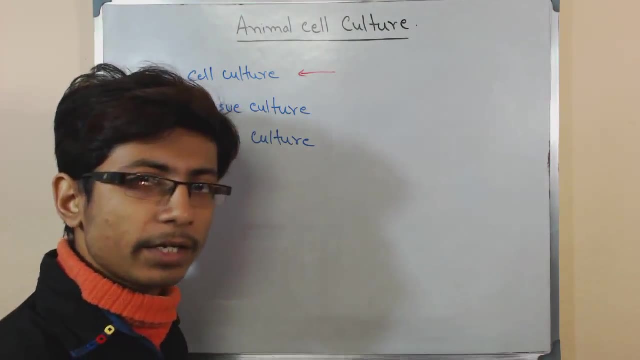 because they're suggesting what they're actually are. you know, cell culture. when you talk about cell culture it means you know in any kind of culture process that we deal with any kind of culture process it means we try to establish a situation in vitro in such a way so that cells or 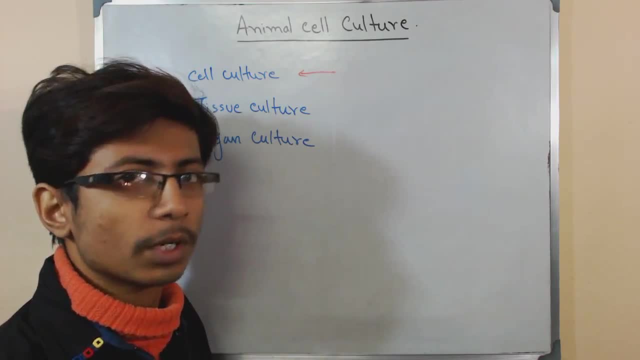 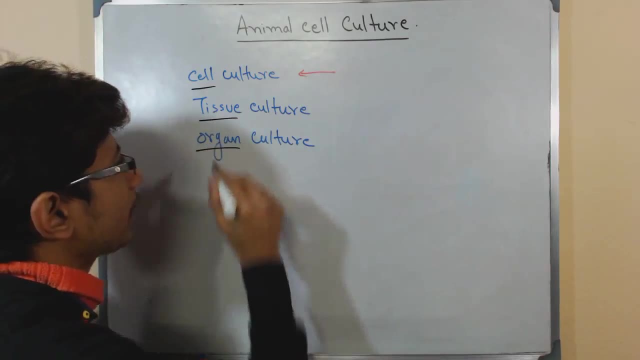 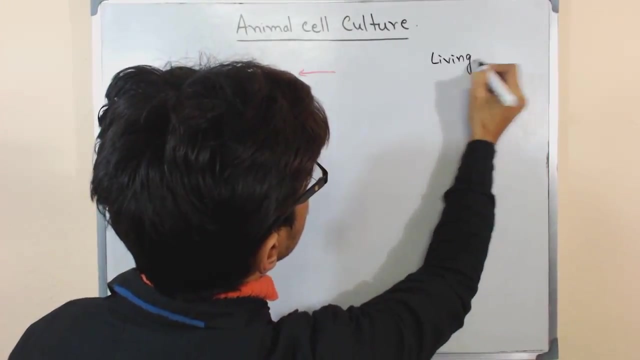 tissue or organ can grow. that is what we are talking about, because you know cells, tissue or organ, whatever we're talking here, all of these materials, you know cells, tissues or organs- they are actually present in a living form, in a living form, in a living organism. right, so we have our living organism now, living organism inside. 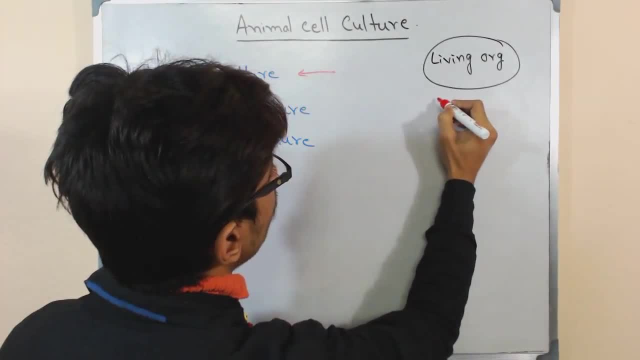 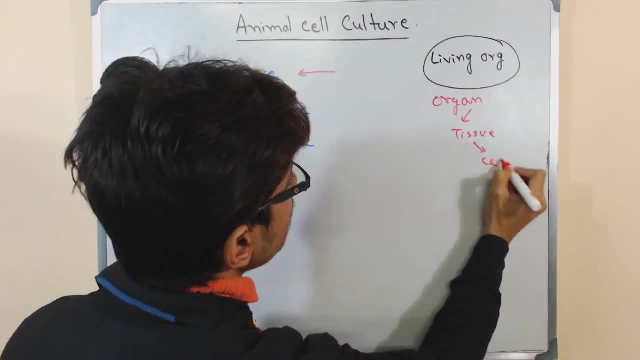 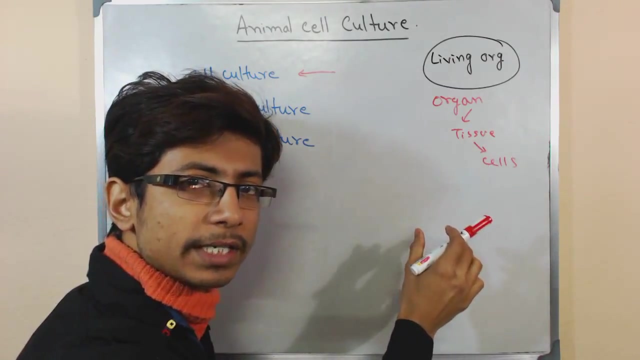 the living organism. we have all of them. we have, you know, organs. if you break down this organ will get tissue. you break down the dish, you will get cells. we're having everything inside right so we, we can take. the cells are the unit organism. we all know that, so we can. 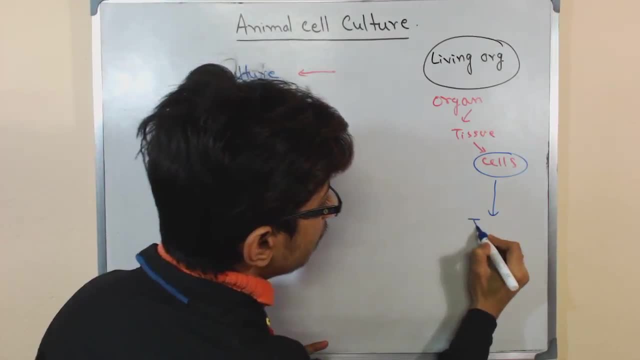 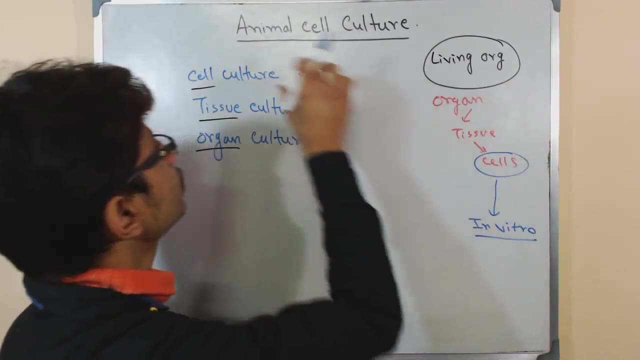 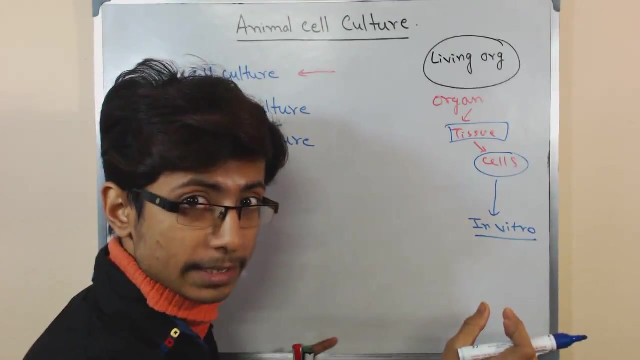 take the unit and take them in vitro and we let them grow in vitro. it convert it into the cell culture. we can take this tissue, which is not the unique part of an eukaryotic organism, but it is made up with cells, right slightly, only more. 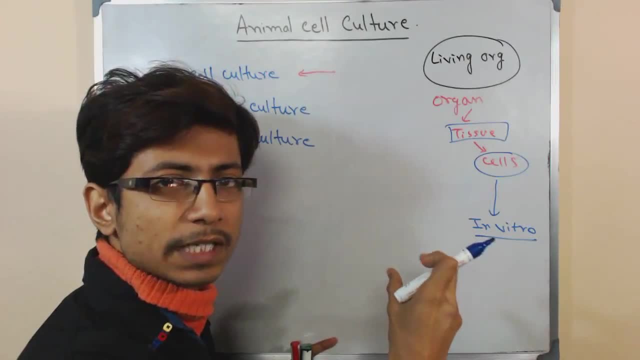 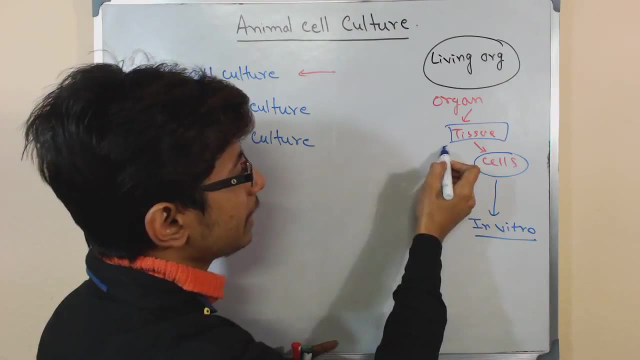 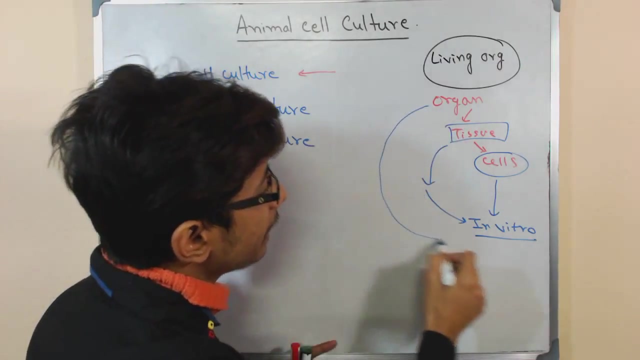 cells have been complete. I mean, say, four or five different types of cells, same types of cells, but number of cells are higher. so say, 50 cells of same type we can take and we can also put in vitro. that will give us tissue culture. we can take the organ directly and we can allow it to grow in vitro. it will give us. 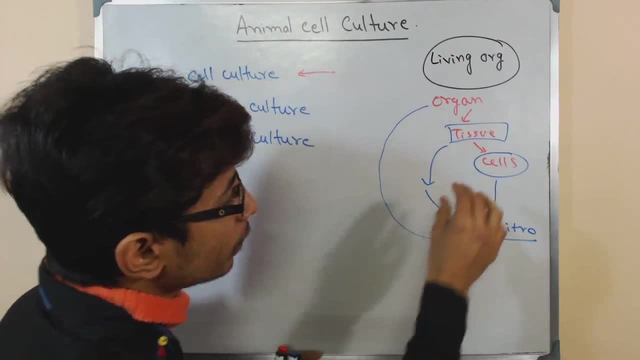 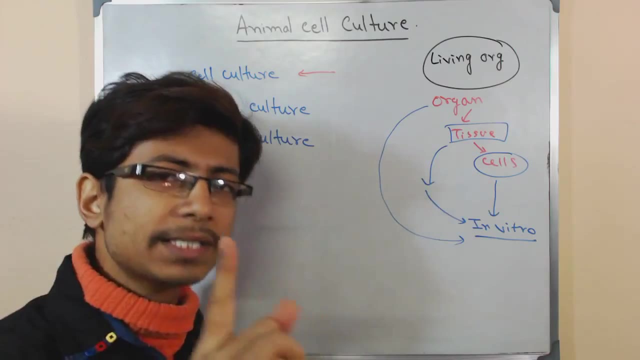 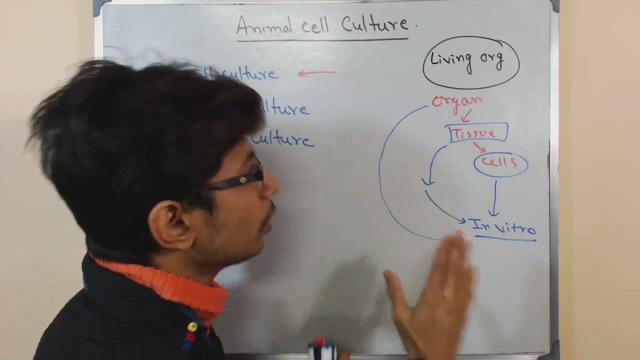 organ culture. but remember, as we going from cells to organs, the thing is becoming much more complicated. because you know, for growing one cell of two cells that you take it's kind of much more easier than growing a whole organ. because you know, if you look at the complexity level of a eukaryotic body, from the unique level to the macro, 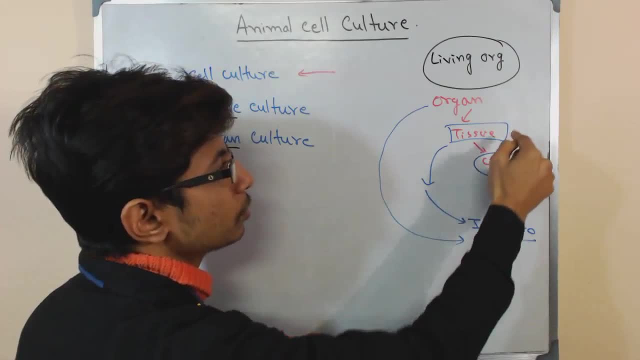 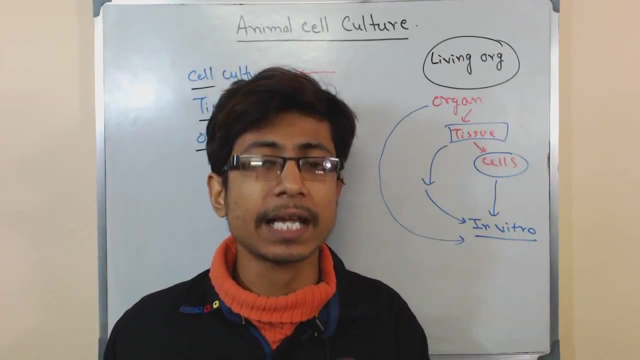 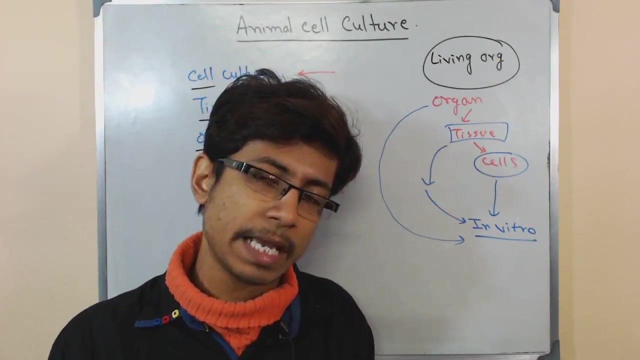 level as we going towards the macro level, from the cell to tissue, to organ, it is becoming complicated, right. so once we are talking about simple cells, cells that produce insulin, we can take that cell, we can grow them in vitro. we have a certain level of complexity now, once we try. 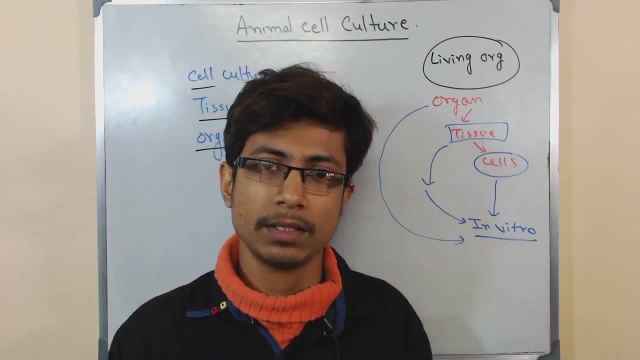 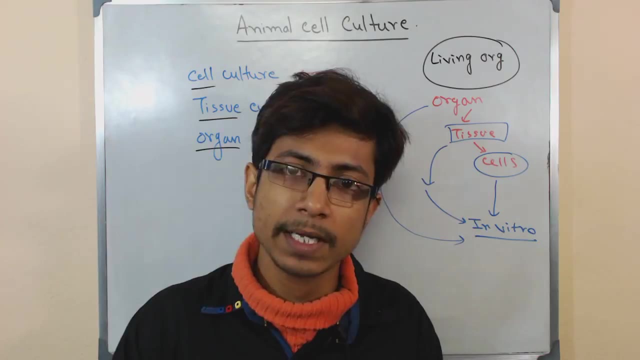 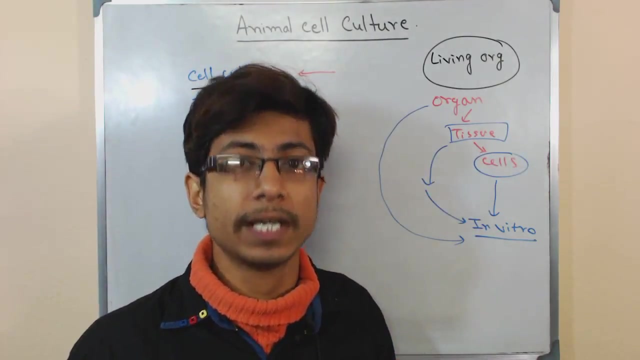 to get some issue that produce that insulin, which in that case the insulin production will be more because we take a chunk off those cells which can produce insulin, in that case the complicit is slightly increases. but now if we take the whole organ that is pancreas, right to grow pancreas in the 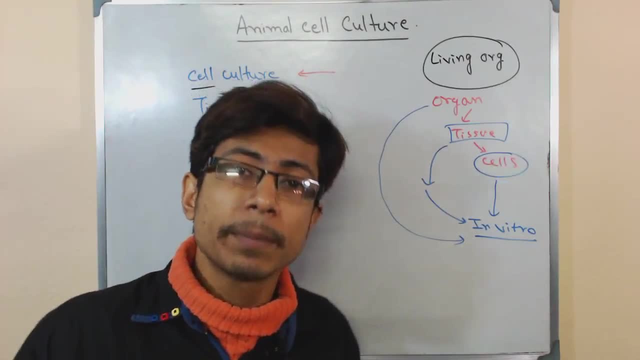 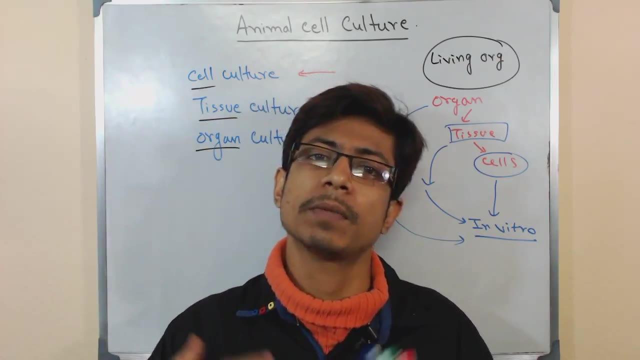 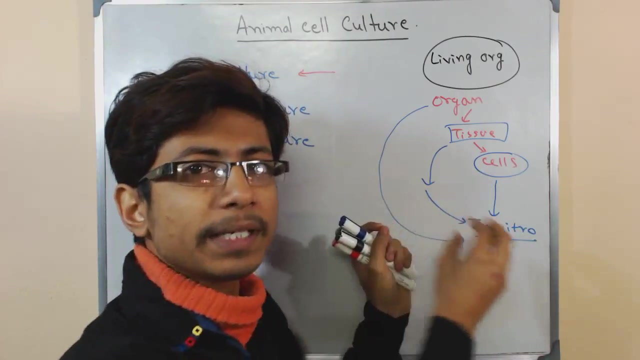 media. in that case the complexity increases because as we increase this hierarchy of physiology, it becomes much more complicated. it because much more thing for development of one cell. the oxygen supply is less right. so the supplement that we need to provide is much more, much, much smaller in case of cells, and it is much 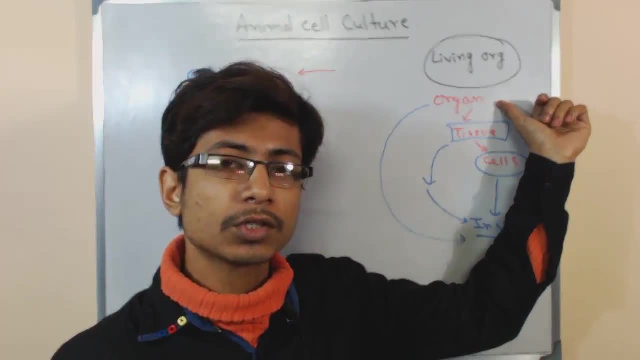 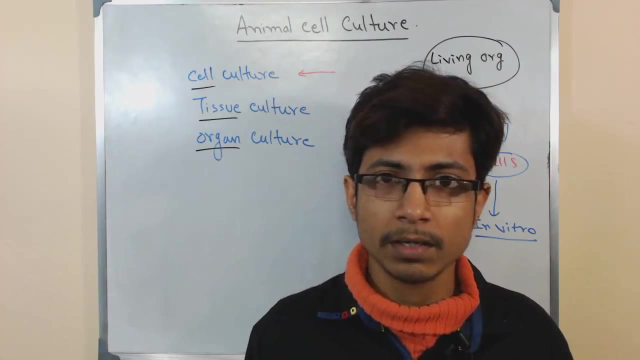 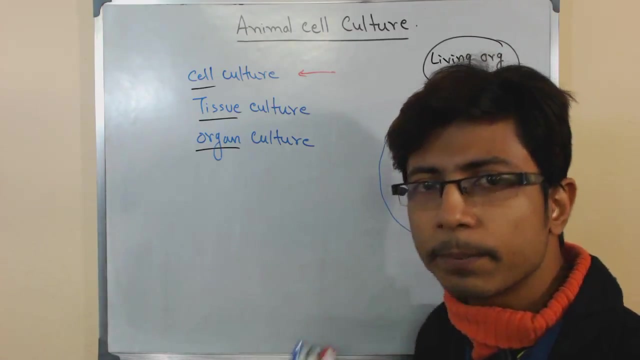 bigger for in case of complete organ growth, right so, organ culture, though there, but still it is much more complicated process and very hard to establish, right? so, if we begin with from the, from the beginning of the cell culture, cell cultures by very basic, because you know we can put them in a- 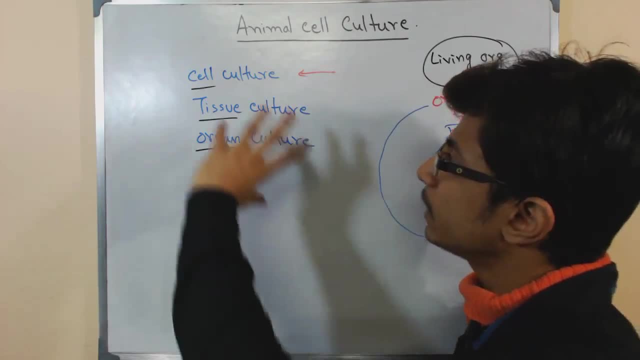 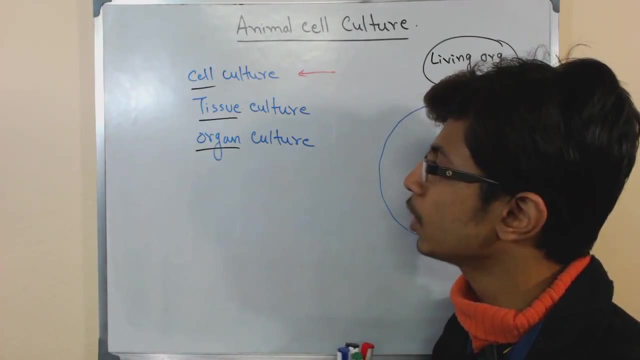 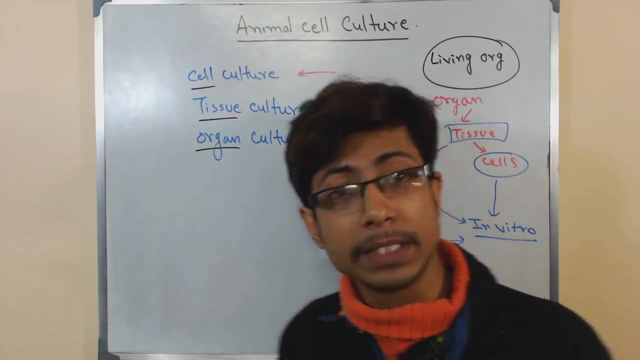 media where we can grow. so the idea is, we are taking the cell or organ or tissue from an individual, from an organism, eukaryotic organism. we put it into the artificial media. right, we are placing them into the artificial media and we allow it to grow. so what should that media contain? that 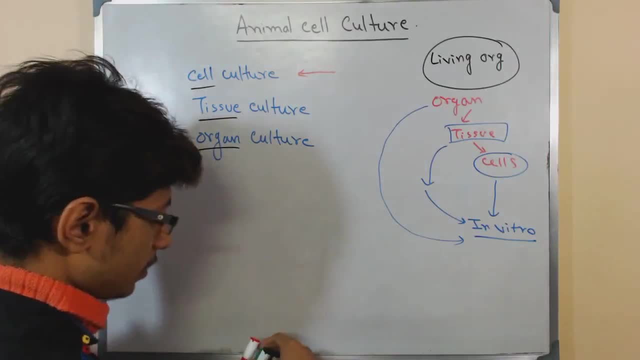 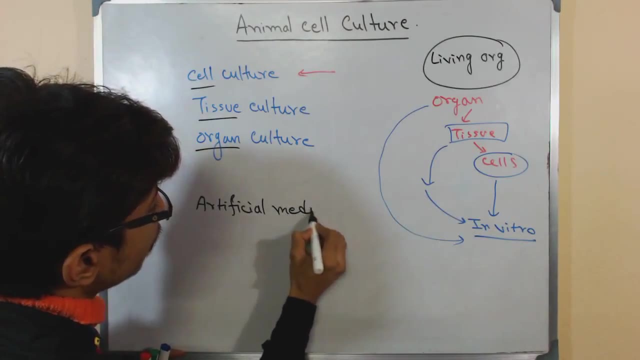 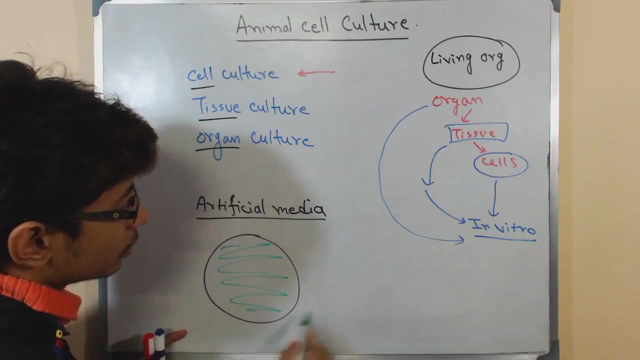 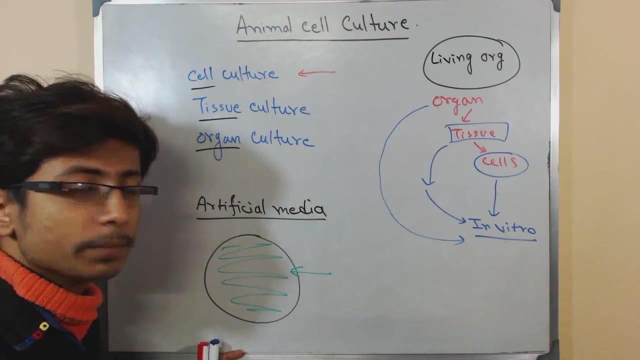 artificial media where we are placing all of these things. let me right here artificial media, saying a petri dish. we are having that artificial media so that artificial media should contain all the necessary ingredients for supporting a cell to grow right, because cells require food and the food for the. 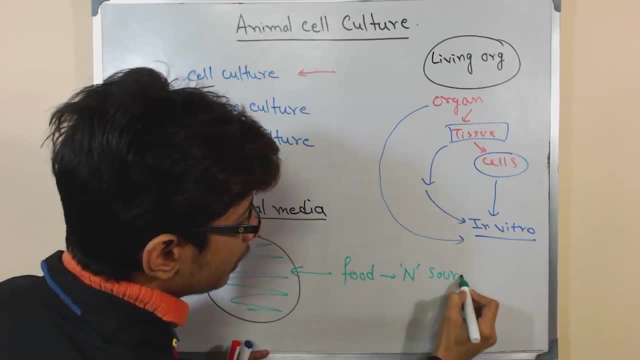 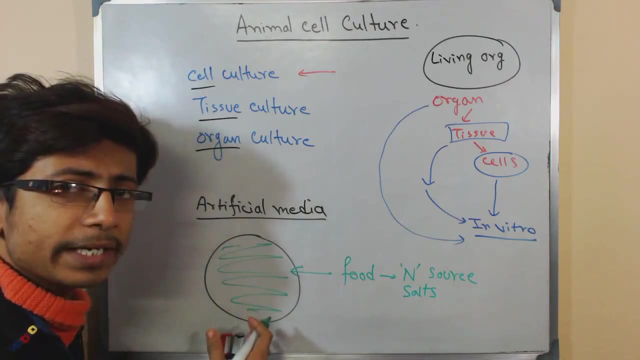 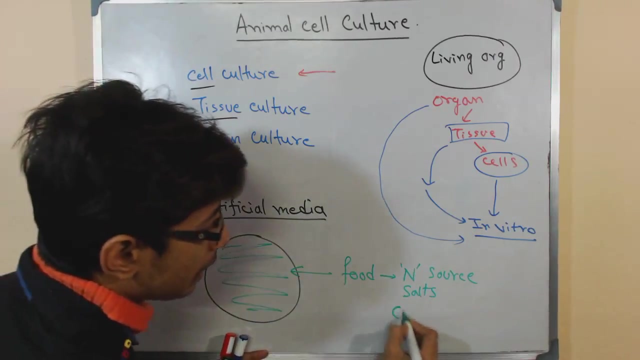 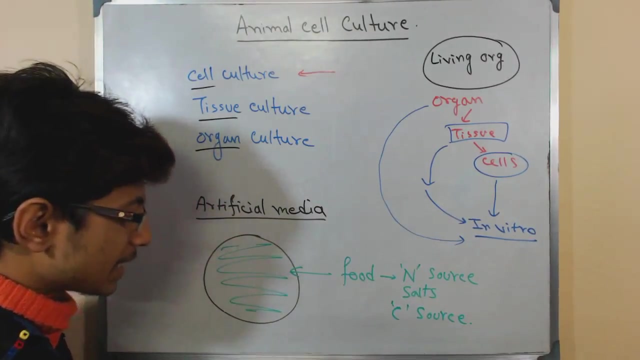 cell will be. nitrogen source should be there right. there should be salt minerals of different kind for maintaining osmolarity and for keeping the other activities of the cell in that there, and also required that we require a carbon source, of course. so these are the food sources that we require in this media, which can support, actually which can support the growth of 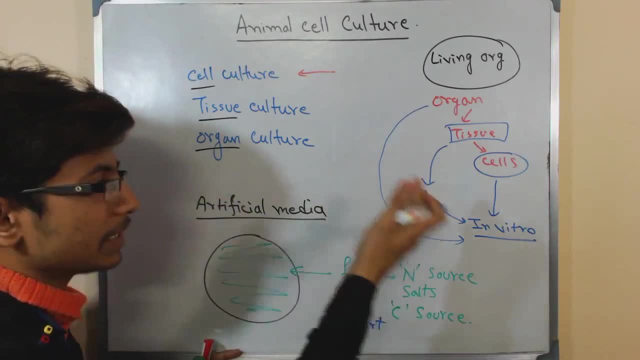 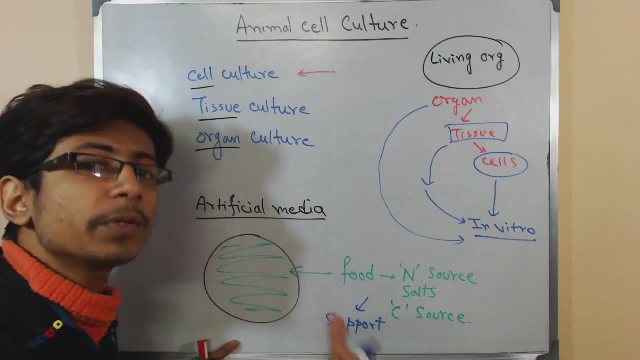 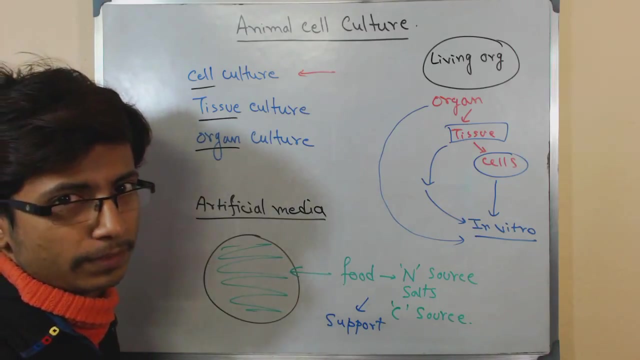 those cells, tissue of animal that we take and put them to grow. these are the features that we require in the in vitro condition and that's what we are creating: in vitro condition for the growth of tissues and cells or organs inside right, but if you are keeping cells only require carbon, nitrogen source salts and all these. 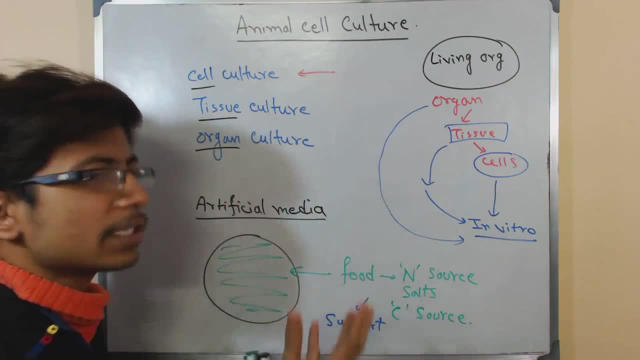 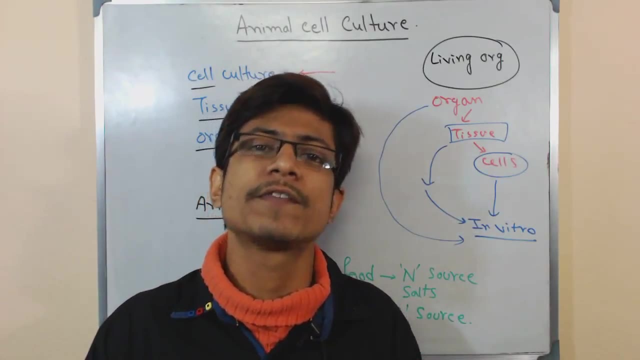 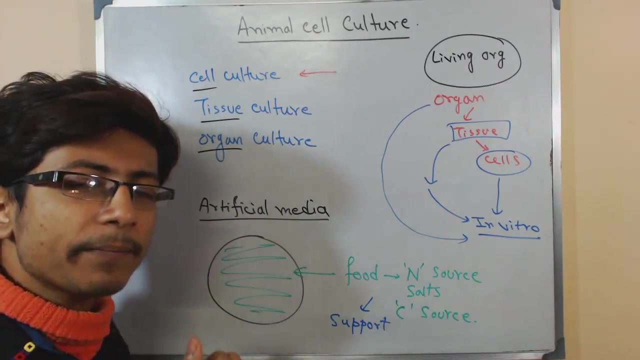 things and it is easy to grow because cells don't require, you know, direct supply of oxygen. in that way we can put the medium in such a way so that oxygen is freely available, so that, say, can take similarly for tissue culture. that is also truly put them into the media. we can make the media, you know we can make. 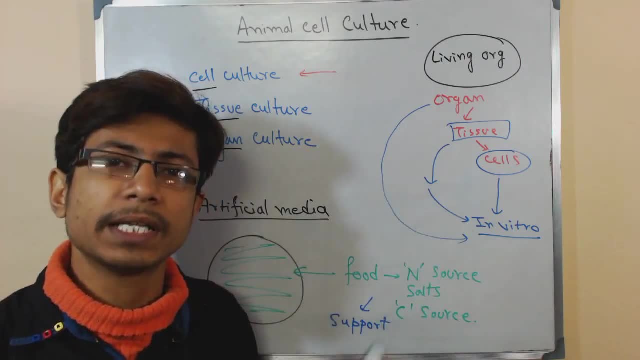 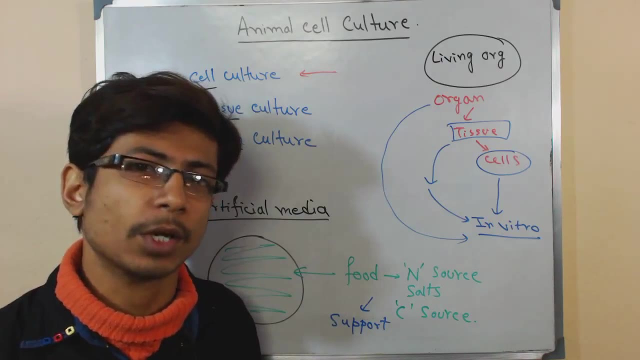 it solid. we can make it liquid generally. the animal cell culture media that we are going to see are, most of the times, a liquid is not liquid. it's kind of semi solid in nature, but not completely solid in that case, because many of these cells tend to grow on the surface.